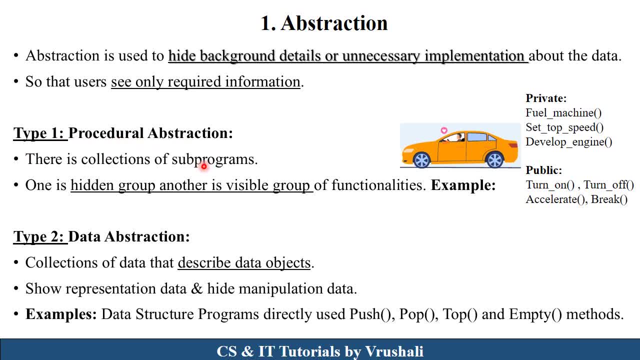 procedural abstraction. Procedural means collections of sub-programs, and sub-programs means there is a collections of two group. One is a hidden group, another one is a visible group of functionalities. Let's see here. I think all of you are familiar with the how to drive a car and how to drive. 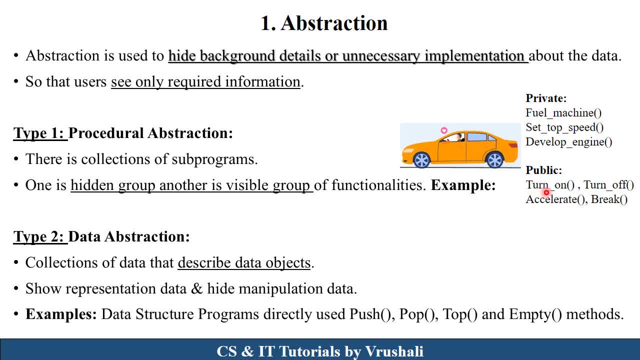 a steps Right. user knows how to turn on the bike, how to turn off the bike, how to apply a brake, how to accelerate the speed. So the user knows this functionality. but the user didn't know how to development of a particular engine, how fuel machine works and how top speed in set Right. So the user 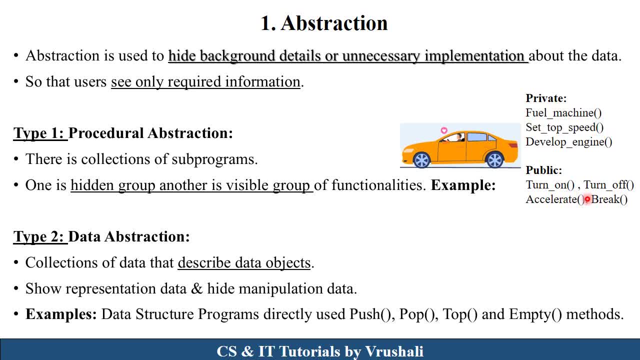 didn't know about this information. user know only required information. so this is called as abstraction. the second type of abstraction is data abstraction. data abstraction means collections of data that describe a data objects. for example, you all are implemented a data structure program. let's take an example of stack program. while inserting element into the string, you can: 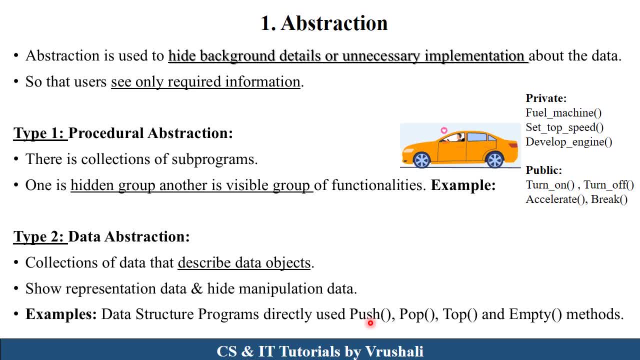 directly use push method, like void push for deleting element from this tag. you can use void pop method, right, so you can directly push pop top, empty this all methods in your program. but you didn't know about how these methods have generate. what was the logic behind those methods, right? 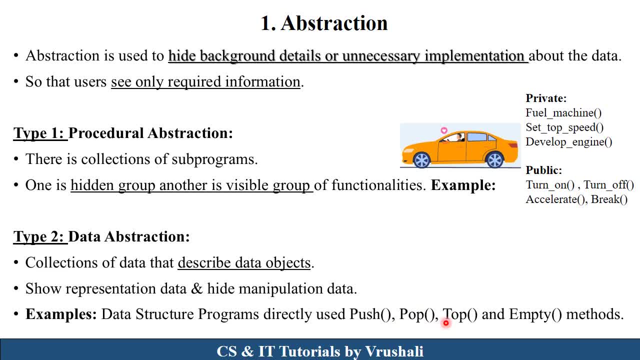 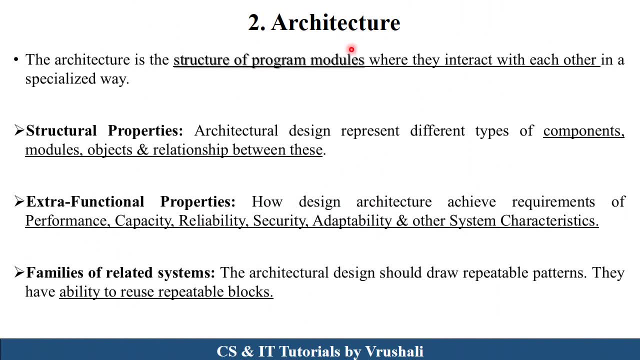 user only related to the front end or built-in information, right, so this is called as abstraction. next now, the next one is a architecture. so basically, architecture means complete structure of the particular product. so it divided into the three parts. the first one is a structural properties. while designing a particular architecture of product, you have to mention all types of components. 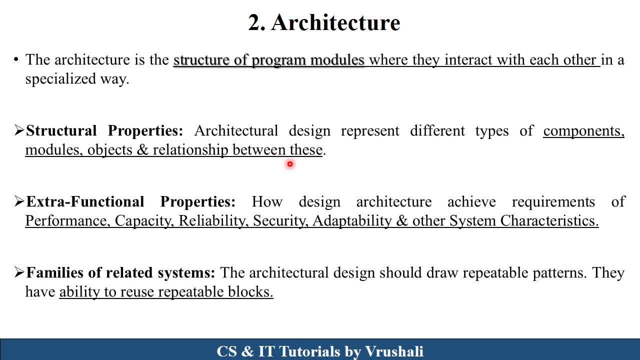 modules, objects and relationship between this. for example, whatsapp application. so in whatsapp there are different modules like chatting module, status module, contact module, then calling module, right, and there are different components have also present. so you have to mention relationship between all these modules and components in design. next one is a extra functional properties. 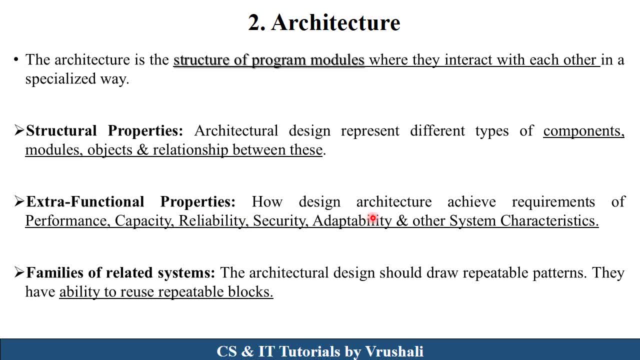 after completing your design. this design fulfill all these requirements, like performance. it shows the performance of particular product, their capacity, reliability, security, adaptability, this kind of features. and last one is a families of related system. see, sometimes you can use the reuse of your code in your product, for example, void display, this function mentioned in one module. 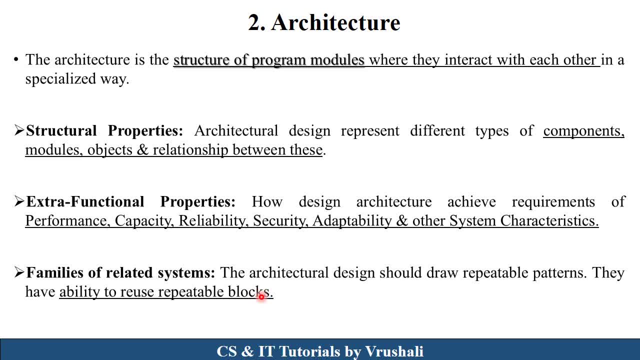 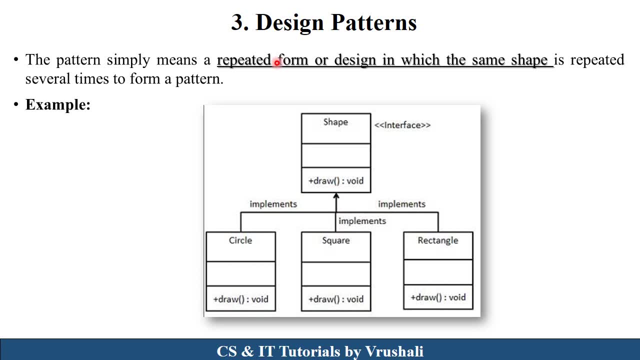 but another two or three module also use the same function, right. so at that time you can reuse those repeatable blocks right. so this is called as families of related system. next, the next concept is design pattern. so basically design pattern means repeated form of design. let's take example: see here. 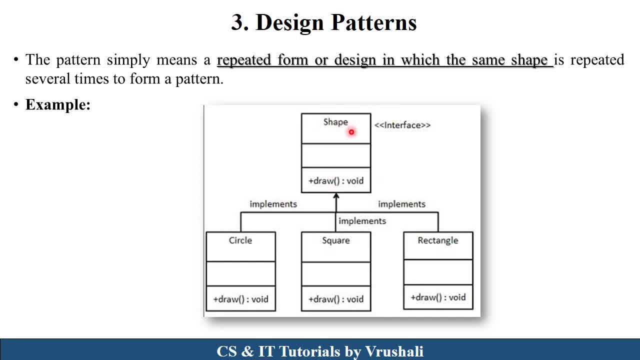 this is a class and the class name is shape. under that shape class there is a method: draw. now this shape class derived from this three classes like circle, square and rectangle, now this circle class also having draw method. so at that time this circle class use the draw method from the shape. 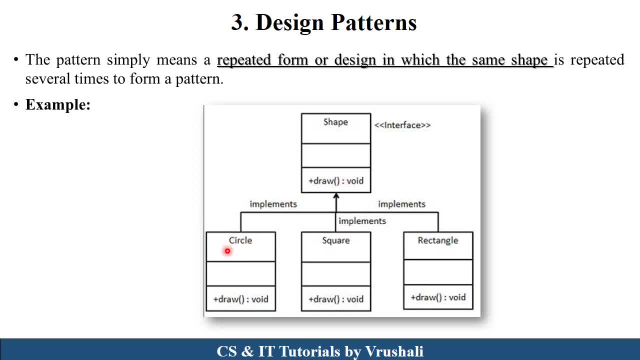 class, because circle class is a sub class of shape class, which is derived from the parent class right. similarly, square and rectangle also having draw method, they also use draw method from the shape class right. so this is a design pattern. there is a repeated form of design, so you can use this method repeatedly several times in the form of pattern. next, 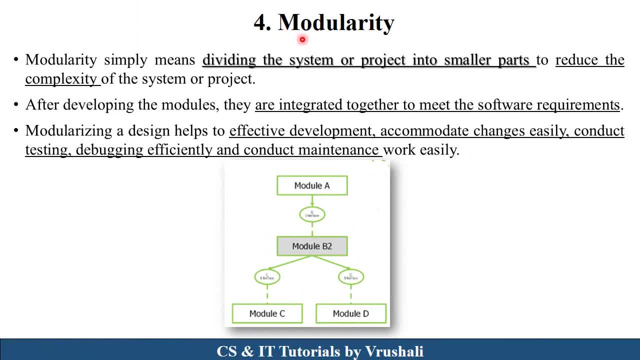 the next one is a modularity. so modularity- the name suggests. modules means while designing a particular product, you have to design a product in different modules. for example, suppose there is a college management system application. now there are different modules. there is a teacher module, under teacher module there is a set attendance, set marks. modules are there then. 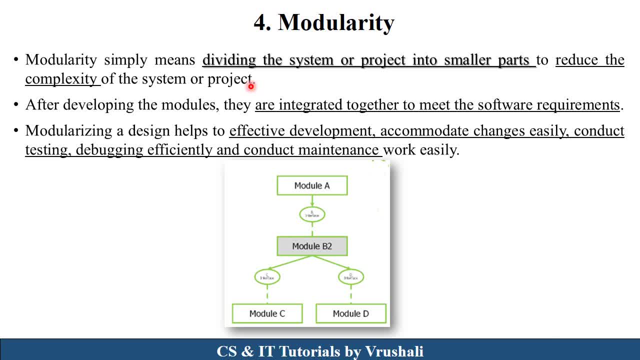 in student module. so under student module there is a gate marks, get question paper. this kind of classes i have there, right. so you have to design a complete product module by module, right, and at the end you have to integrate all those module and check that whether it is meet the customer. 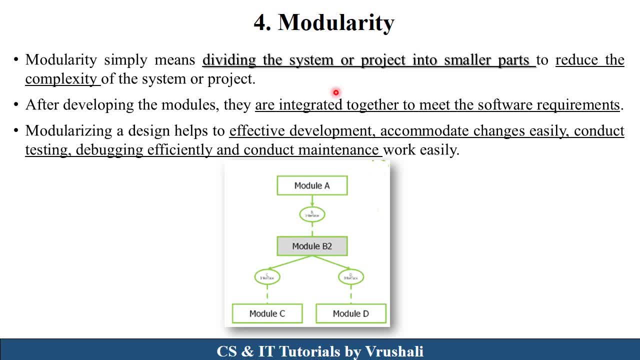 requirements or not. the advantages of modularity is there is a effective development. right then accommodate changes easily. if customer want any changes, you can do this. particular changes in specific module, not a complete program. right then conduct testing and debugging efficiently because module by module development, and also conduct maintenance work easily. 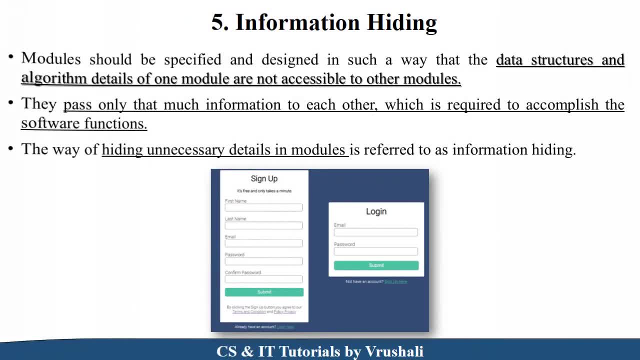 so this is called as modularity. next, now, the next one is a information hiding. so basically, while designing a particular product, you have to design module by module, right, but at that time you have to take care of this thing, like all the informations not shared with all the other modules means, for example, data structure and algorithm. 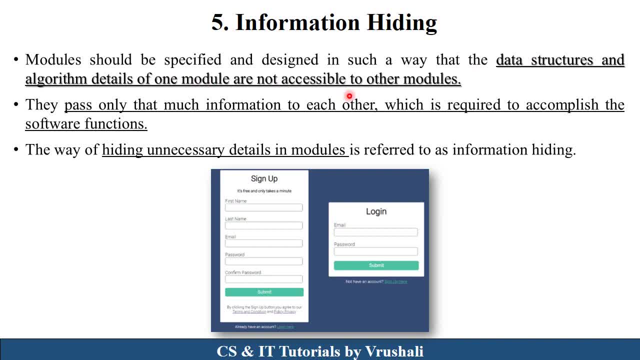 details of one module which is not accessible to other module or only required information are accessible to other module, right? just see here in this example. suppose this is a signup model. in signup model you have to enter first name, last name, email password and confirm password and you have to click on submit button right now. next step is login. 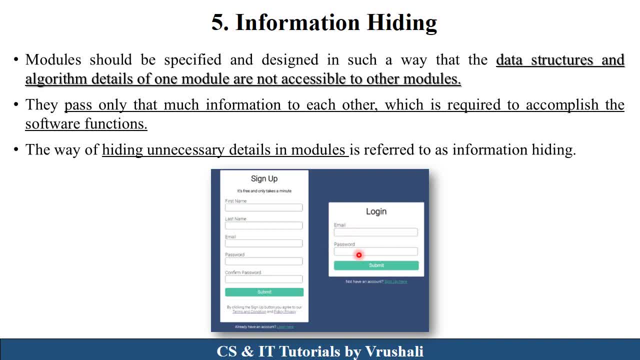 so login purpose, you just required email and password option. right? you can't require first name, last name. this kind of information means this login module share only required information from signup module and all the unnecessary information are hide from this login module. so this is called as information hiding, that is, hiding unnecessary details from the model. 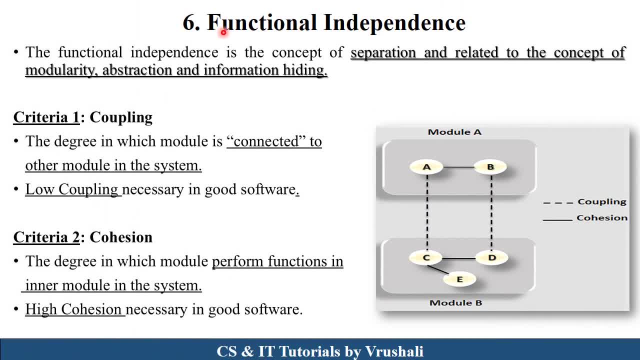 clear next now, the next one is a functional independence, so generally functional independence, which is related to the modularity, abstraction and information hiding concept. see here there are two type of criteria: criteria one is coupling and criteria two is cohesion. let's see here, in this particular diagram, this is a module a. in module a there are two classes, class a and class b. now in 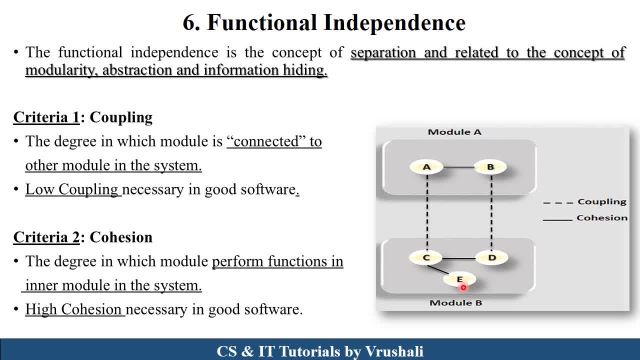 b. again there are three classes: class c, d and e. now the a class from module a access information from c class of module b. right, so this is a intra connected. this is called as coupling. okay, but now in cohesion, which is interrelated, means a and b. these classes share the information. 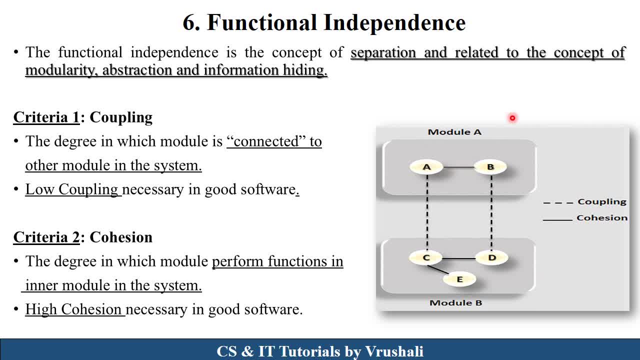 so this is called as cohesion. cohesion happen intermodule, but coupling happen them. when they access data from another module, they access information from one module to another module. right, we discuss this coupling and cohesion in detail next session. okay, so basically you just remember this thing: coupling provide connection of one module to another module. 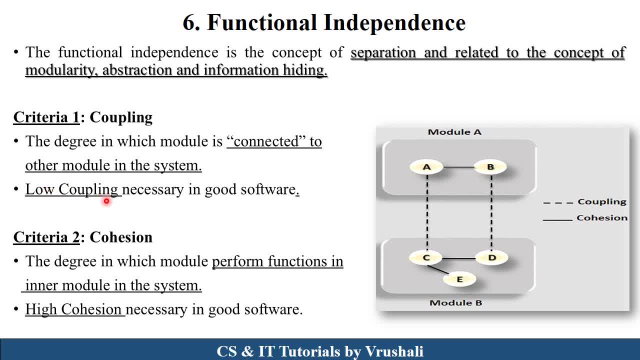 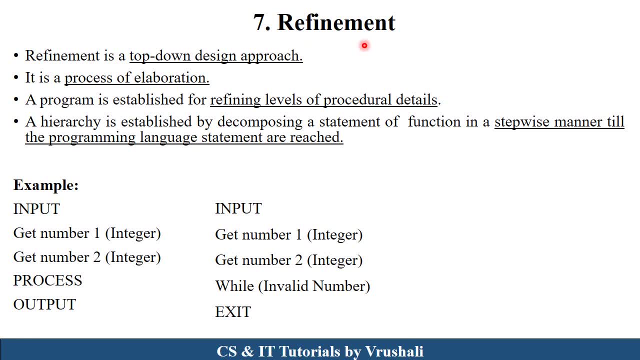 and cohesion perform the function within the model right. so for generating a good software design you have to require low coupling and high cohesion. next, next, now, the next one is next is a refinement concept. so basically, refinement is a top down design approach and it is a process. 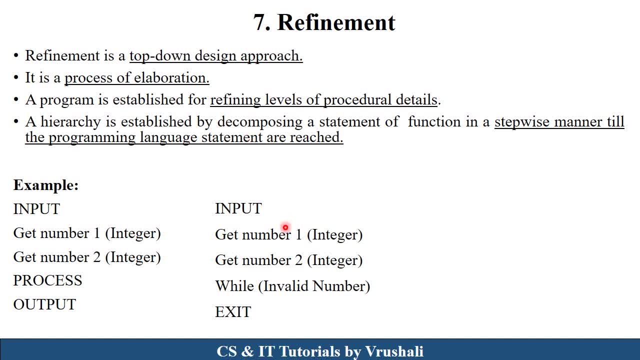 of elaboration. just take an example here: while complete your program you perform the compile and run this kind of functionality. okay, so after running your program, just take an example here- suppose you have to perform addition program. so after compiling your program- the first one- you have to take a input on compiler like enter the first number, that is, gate number one, then enter. 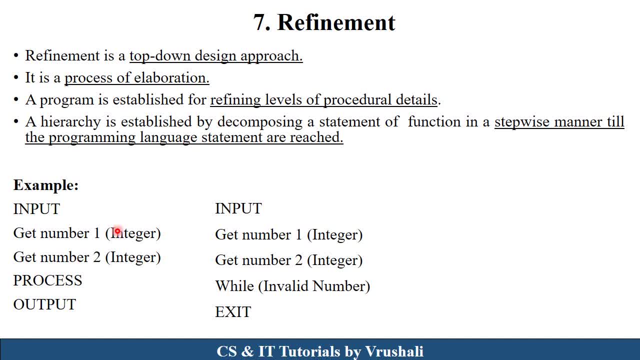 the second number, that is gate number two. suppose first number is four, second number is four. in process they perform the addition like four plus four, eight and display the output eight. right after that you have to again perform the addition which take a input like gate number one. suppose 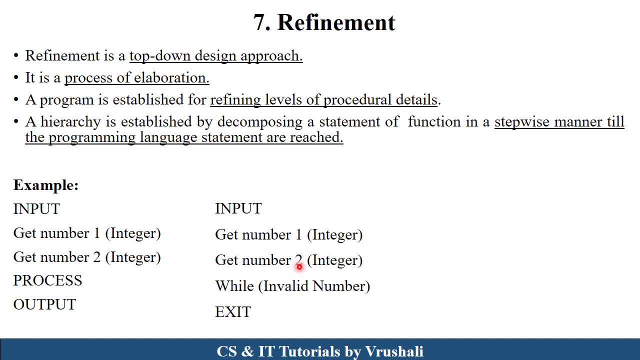 first number is two and gate number two. so at that time you have to bi-mystically enter a, only a value, that is string value, but two plus a. it is not possible, right? so it generate a while that is invalid number is there and they exit the operation, right? so this is called as refinement- refinement. 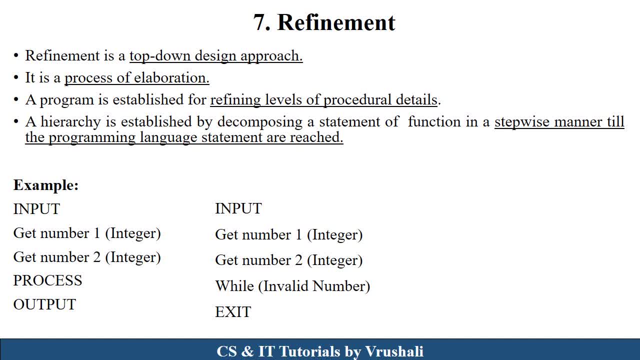 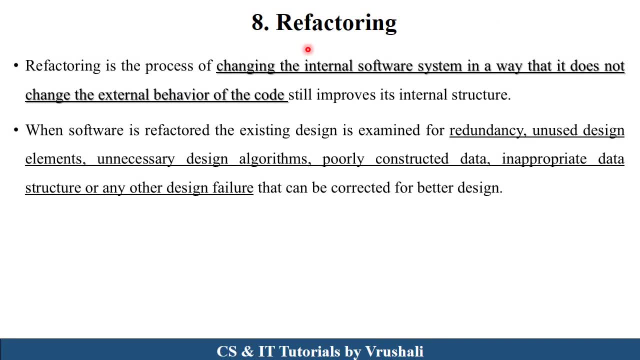 means stepwise manner, stepwise execution of particular program and stepwise execution of particular algorithms. clear next. now, the next one is a refactoring. so the concept of refactoring is while you make any changes in internal software which is not affect on external behavior of the code. this is called. 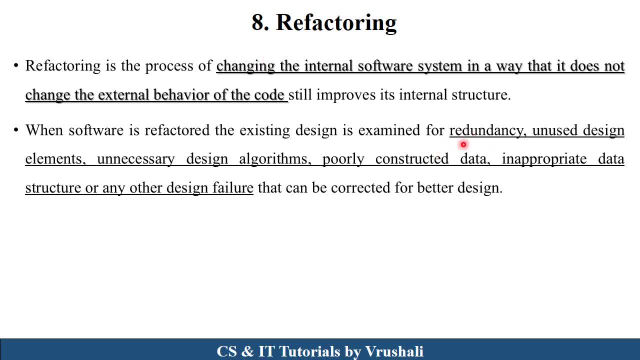 as refactoring. just see here. suppose you have to remove duplicate data in internal system. you have to remove unused design elements, unnecessary design algorithm in internal software. you have to also remove some inappropriate data structure in poorly constructed data information. so after removing all those thing, which is not 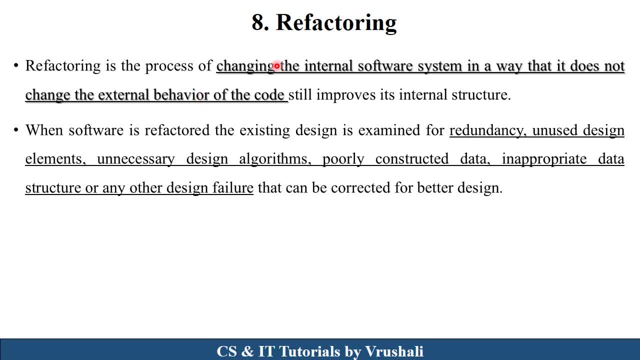 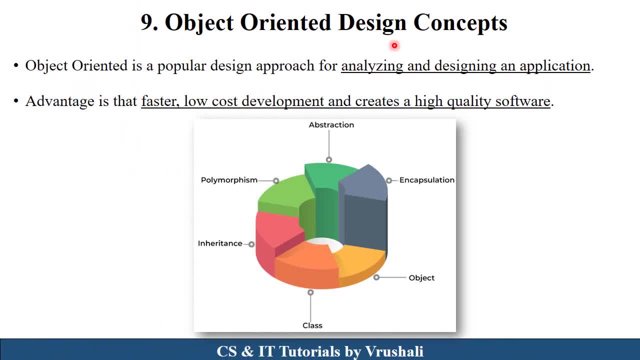 effect on external behavior of the code, right, so this is called as refactoring, which generate a better design. next, and the last one is object oriented design concepts. i think you all are familiar with the oop concepts. so here, object oriented concepts, there are class, that is, 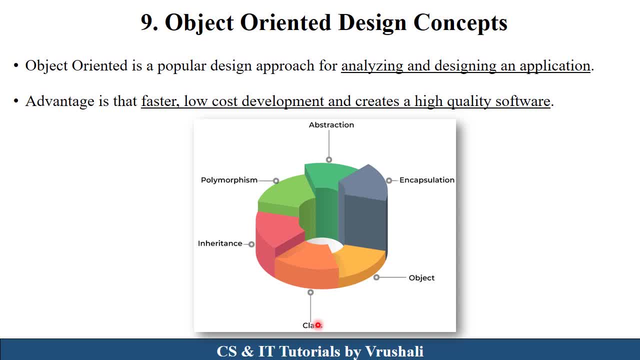 collections of different objects, methods, functions, then objects, inheritance. inheritance means suppose there is a parent class, like there is a student marks. this is a parent class under student marks. there are different child class, like class test marks in same marks and same marks, right this all are the child of the marks class. so this parent child relationship shown in inheritance. 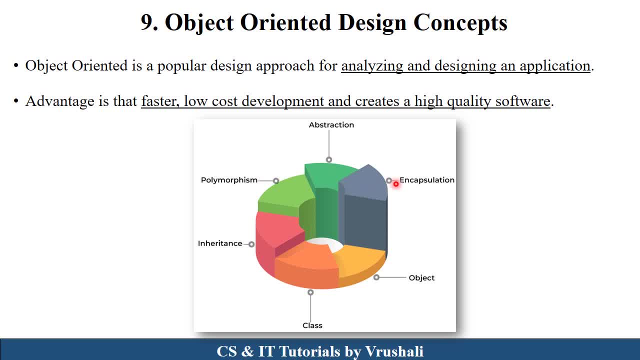 then abstraction, polymorphism, encapsulation, that is, collections of same types of classes and methods are there. so these all approaches have implemented, while generating a good design of particular product and, due to oop concept, it shows faster and low cost development and create high quality softwares. 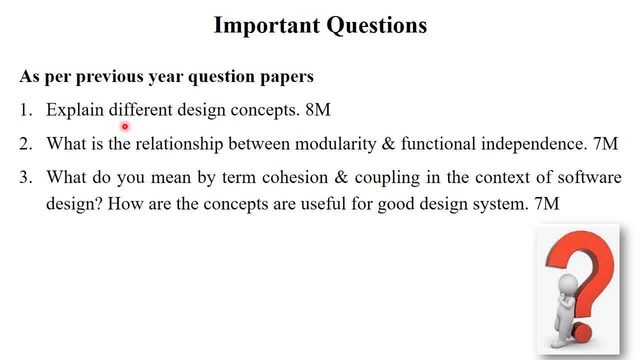 now on this particular topic in previous year question paper. it asks: explain different design concepts for eight marks. then what is the relationship between modularity and functional independence for seven marks? here modularity means just divide complete product into the different modules, but functional independence means the relationship between all those models, right? 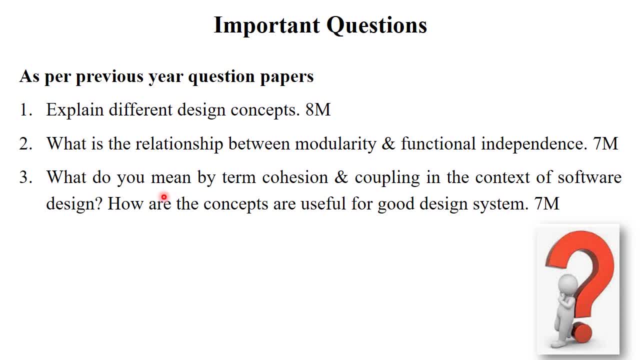 and this is the concept of oop concept. it shows faster and low cost development and create high quality software. this question, this is one of the most important question. what do you mean by term cohesion and coupling in the context of software design? how other concepts are useful for good designing? 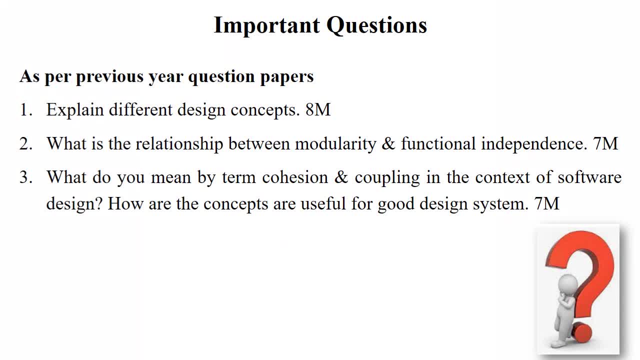 system for seven marks, so you have to prepare all these questions. this is all about design concepts. thank you, keep learning.